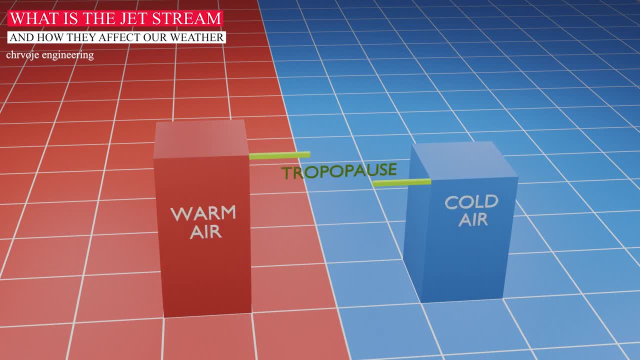 defines the topography of the jet as follows. The tropopause defines the topography of the jet at the X area and the top of each column. A shorter column of cold air has the same surface pressure as a taller column of warm air. This is because in the cold-air column 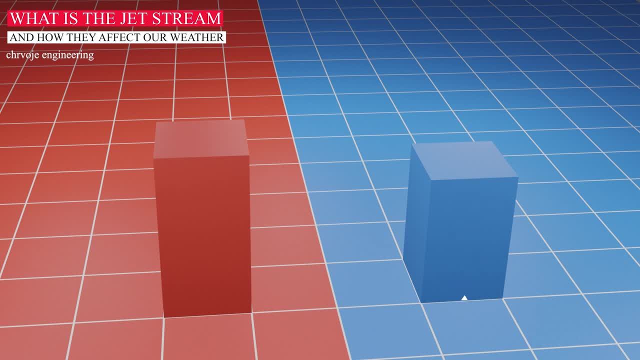 the air is more dense. This causes atmospheric pressure to decrease more quickly with heights. In the warm air column, pressure does not decrease as rapidly with height. because the warmer air is less dense, The tropopause in both columns is at the same atmospheric pressure. 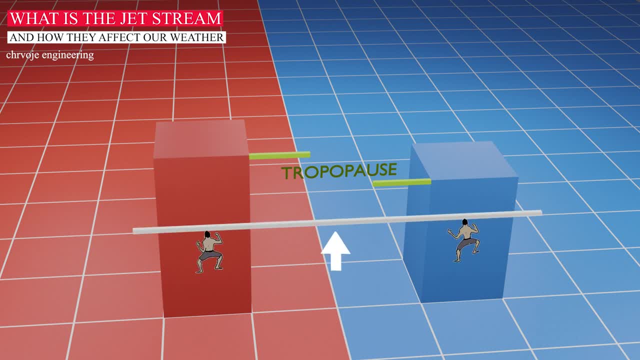 So if you climb to the same heights in both columns, you would discover that the cold air column has lower atmospheric pressure, while the warm air column has greater atmospheric pressure. The pressure difference caused by this temperature gradient produces a pressure gradient force. The pressure gradient force acts from high to low pressure, so theoretically, 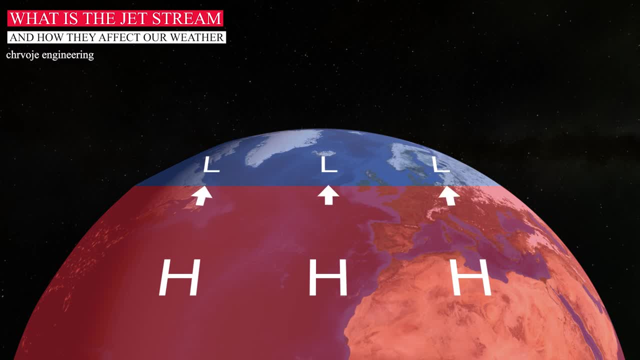 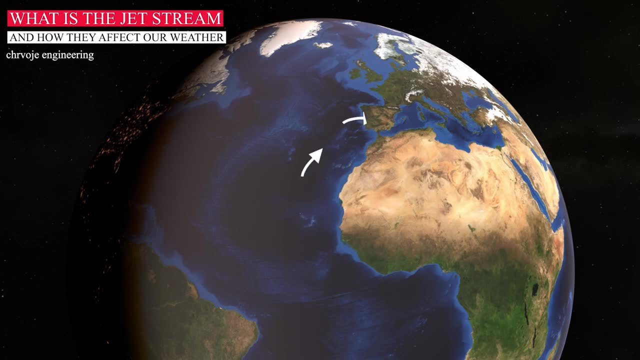 in the Northern Hemisphere air would flow from south to north, But the Coriolis force resulting from the Earth's rotation causes the air to move to the right of the direction of motion in the Northern Hemisphere and to the left of the direction of motion in the Southern Hemisphere. 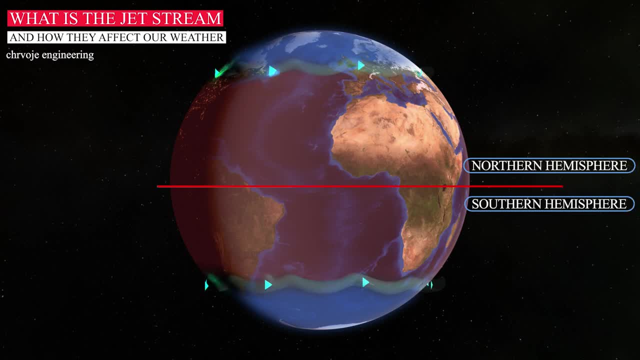 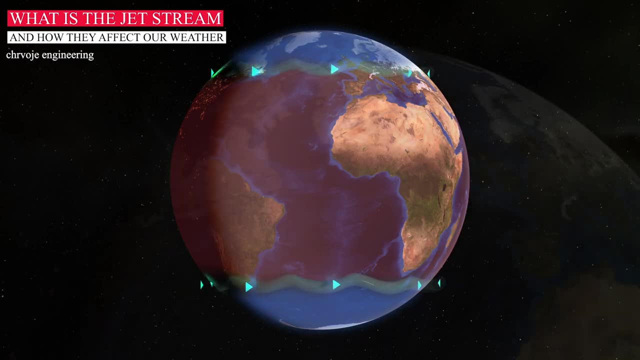 The jet stream travels parallel to temperature gradients in both hemispheres, flowing from west to east. Theoretically, this jet encircles the Earth in a condition where the temperature is or does not reach 100 ° C continuous line, But in reality it is more broken up as differential heating of land-sea. 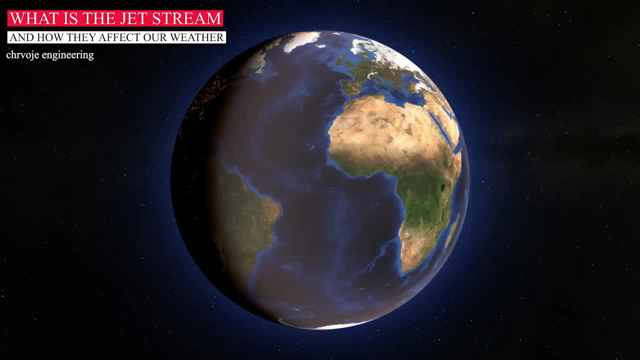 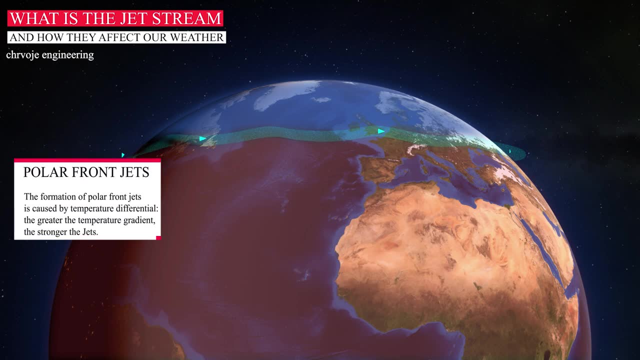 masses lead to west-to-east temperature contrasts as well as north-to-south. The formation of the polar front jets is caused by temperature differential. The greater the temperature gradient, the stronger the jets. This indicates that the jet is more powerful in the winter than it is in the summer, as the Earth poles cool during the winter months. 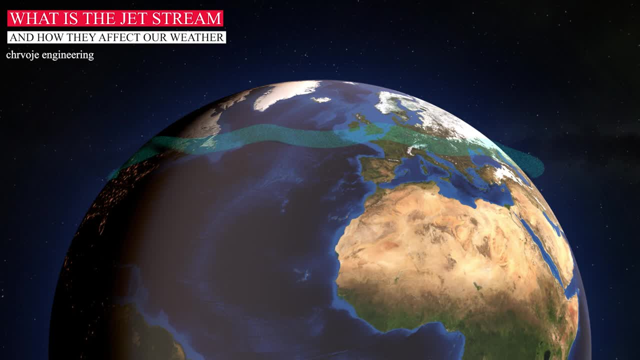 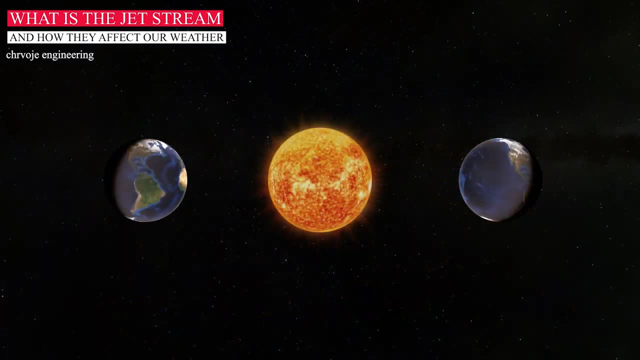 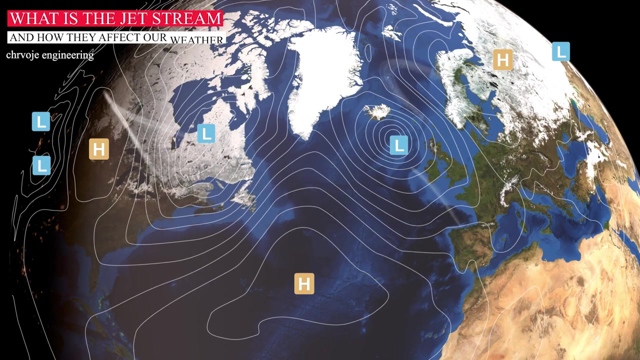 increasing the temperature contrast. In the Northern Hemisphere, the jet tends to be further south in winter and further north in summer. This is due to the incline of the Earth and that in winter the Northern Hemisphere is inclined away from the Sun and in the summer it is inclined towards the Sun. Mid-latitude low-pressure systems occur on.